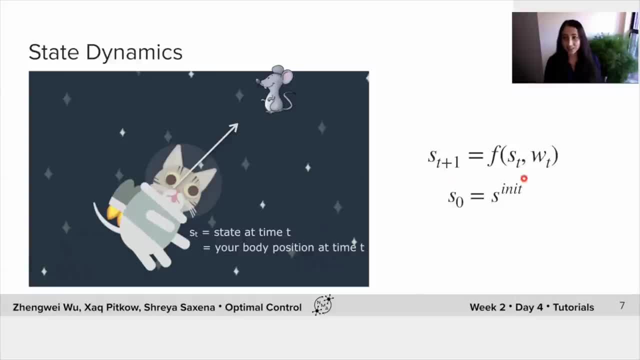 any action on it. In general, these state dynamics can be a nonlinear function. Here f is a nonlinear function of your state at the last time point and of the noise. Now that becomes very tricky mathematically. So in this tutorial we'll consider that your state is a linear function. 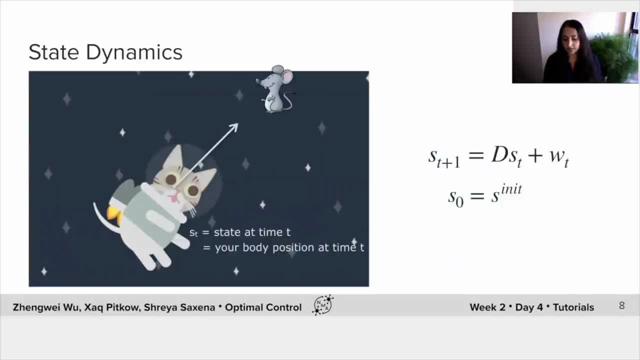 So you can see that the state is a linear function of the state at the last time point and an additive noise term. So, as I said, this is a linear function and this is a good approximation for a lot of dynamics. Now, as I said, this noise, this process noise it's called, this is any kind of 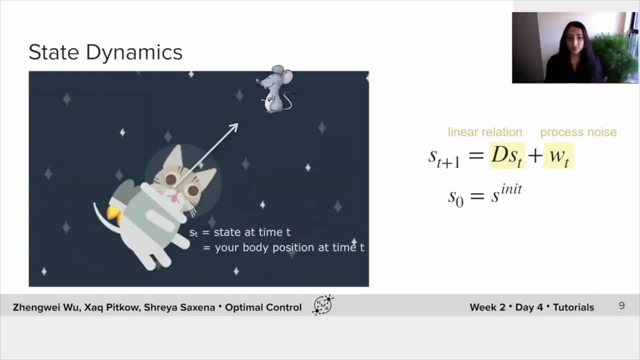 environmental noise that may be affecting you. that cannot be modeled, So in this case it could be meteorites hitting you and changing your body position from in an unexpected way. So you can see that the state is in an unexpected way And we'll start off with an initial condition. 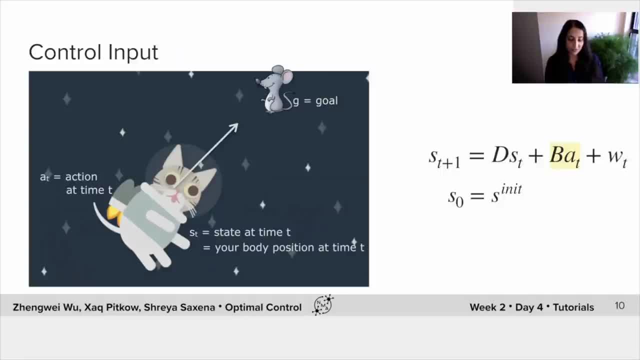 Great. So of course, you want to get to the goal of the number. So this is the action that you apply in order to get to the goal. This action also linearly adds to your state dynamics. So any action at time t, one unit of action at time t, will create b units of. 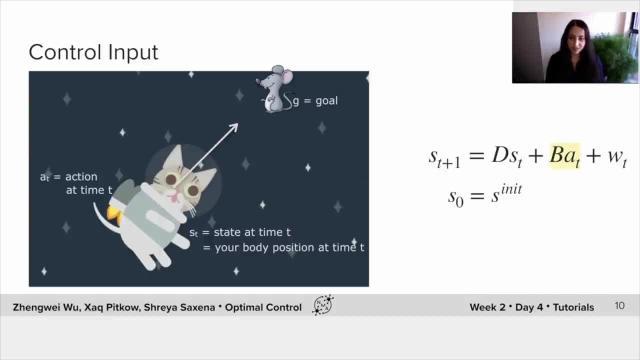 b units of action at time t plus one. Okay, so these are the dynamics that we're considering, And the question now becomes: how do you actually optimally design this action at time t or at all times, in order to reach this goal that you want? Okay, so let's start with something called open. 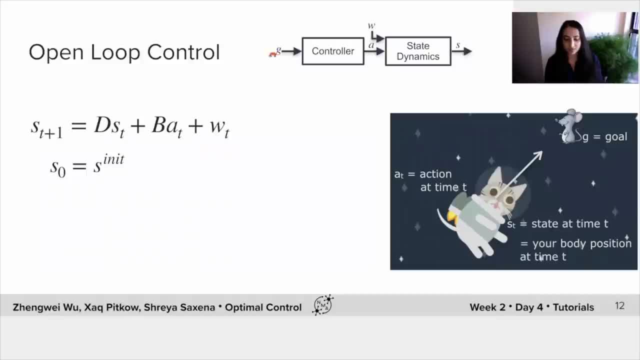 loop control. Here I'm just drawing a block diagram for what these equations entail, And so just to get an intuition of how we can actually start designing this action in order to reach our goal, I'll go through an example with some numbers. So this is what we want. 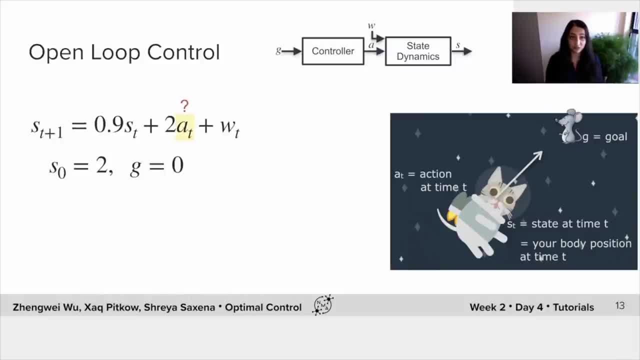 we want to design this in order to get to our goal. So let's consider: our goal is at the origin, So this mouse is at the origin and we have been displaced at some two units in order to- and we want to get to the origin. So in this case, what we would do is we would, we 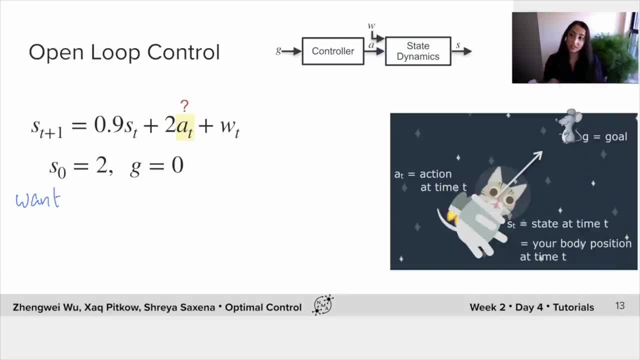 want, let's say, to. let's say we would want to get to the goal in one time step. So we would want: S1 equals zero. Now, what is S1?? It is a linear function of your last state, plus a linear function. 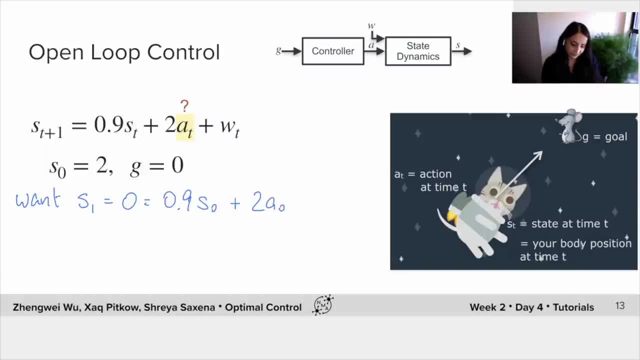 of the action that you will take at time zero And in general. of course, it's also a function of the noise, but we are going to, for this example, just consider that there's very low noise. We're looking with no linear rights around. Okay, So we want this, Let's plug in. 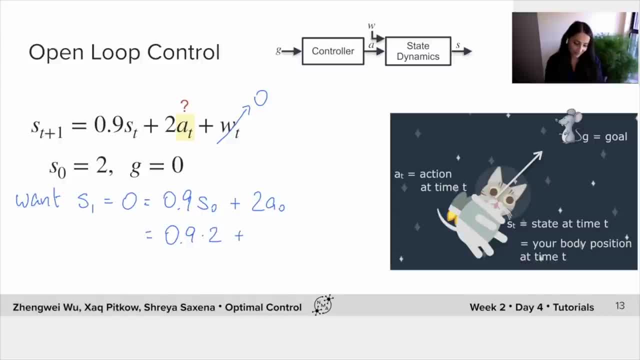 of course, our state at time zero, And what we want to find is this A0 such that S1 is equal to the goal, is equal to zero, And we very easily find that the optimal A0 for that is just negative 0.9.. Great. So we want to apply negative 0.9 of action in order to get to our goal and just get to the goal. So we want to apply negative 0.9 of action in order to get to the goal. So we want to apply negative 0.9 of action in order to get to the goal and just get to the goal. 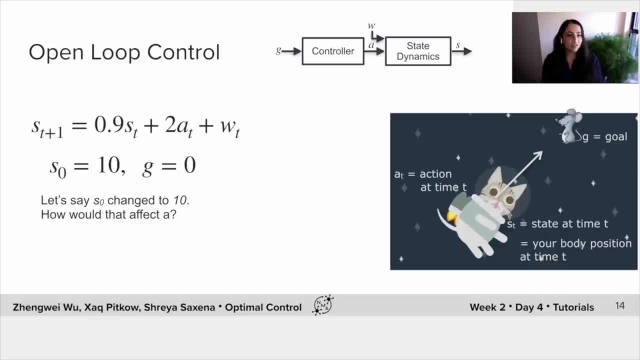 So we want to apply negative 0.9 of action in order to get to the goal. So what happens now if S0 actually changed to 10?? So let's say you're further away from your goal because you've been displaced further. How would that actually affect your action? Well, it's easy to find out. 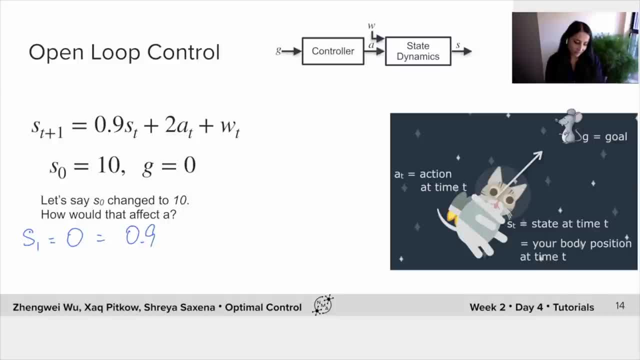 Let's say you still want to get there in one time, step right This time. your desired state at time zero is a function of your current state and we, we can just again assume that this noise is negligible and solve in order to get your. 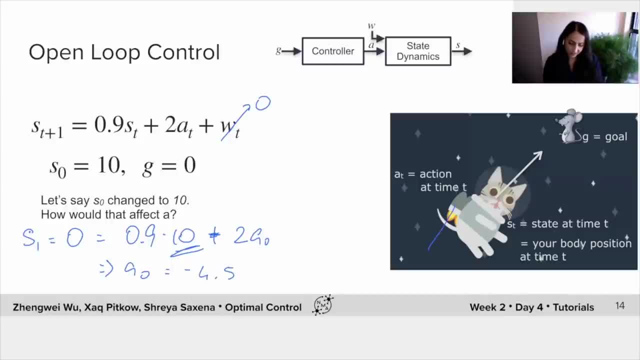 optimal a0 is negative 4.5. so you'll see, you'll just need to apply a much bigger action in order to get to the golden one-time step. that makes sense, great. so you'll notice that the desired a, the desired action, actually changes depending on s0, the initial condition. this makes sense. 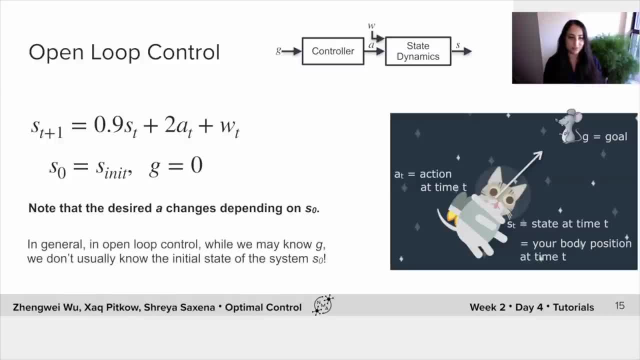 um, but the problem is that in open loop control, in fact, while we may know g, the goal, we don't usually know, uh, the, the initial state of the system. s0. we may know the dynamics, but we don't know, uh, the state itself. and this creates a problem because even if you, now you know, apply, 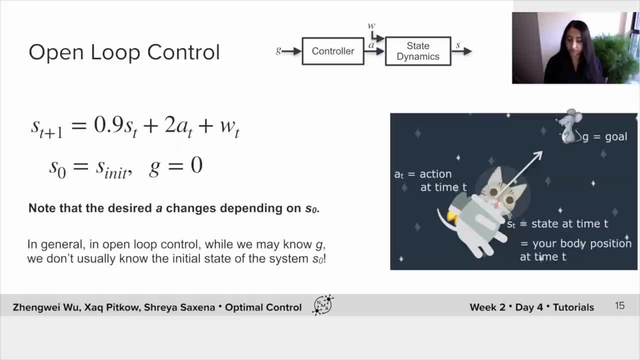 a suboptimal a of t for a couple of time steps in order to get to your goal. somehow, you um are still affected by the state of the system and you don't know the initial state of the system. and you don't know the initial state of the system and you don't know the initial state of the system. 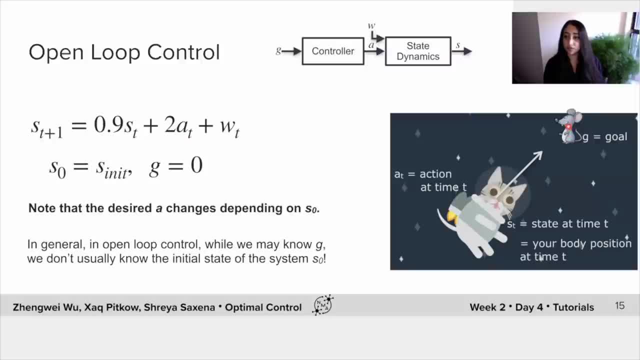 so, even if you get to your goal, you may be knocked around, uh, around your goal. um, let's say, like going circles, or just be, um, drift around the goal. you can't do anything about it. um, so this, this does create a problem. uh, how do we fix this problem? in fact, we can do something called closing the loop. 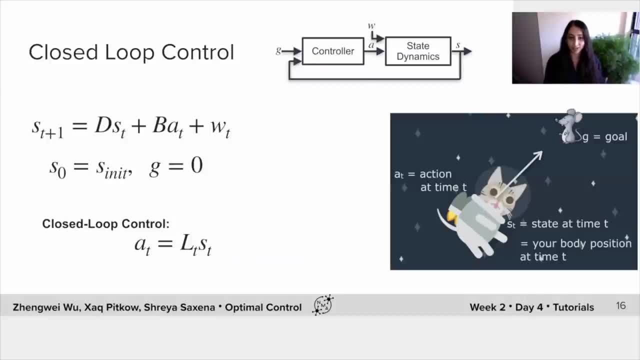 so here i'm closing the loop, and this is called now a closed loop controller. um, you can see, in fact, open loop control as one extreme where we may not know anything about the position, and closed loop control is, in fact, the other extreme where we know the position exactly. 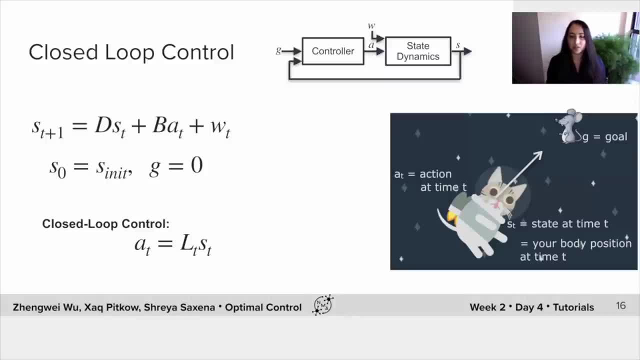 later on we'll see a more realistic case where we have partial observations of the state and we still have to make an action. but here, our action here has uh access to our state at time t. in fact, we formulate it as a linear function of the state at time t. so this is the state of time: t is multiplied by something. 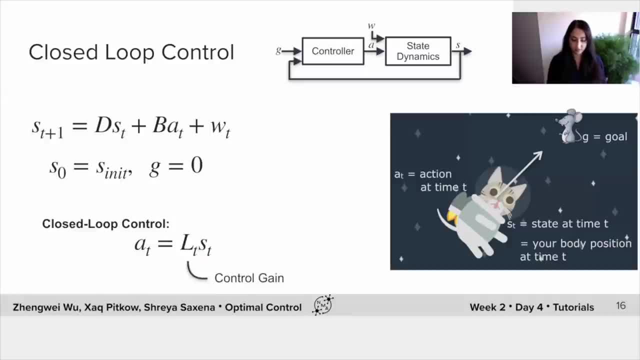 called a control gain, in order to get our our action. so how do we now design this control game? so that's what our problem is coming out of: design the control gain in an optimal, in an optimal way, in order to get to our goal. so so, let's get back to our numbers. 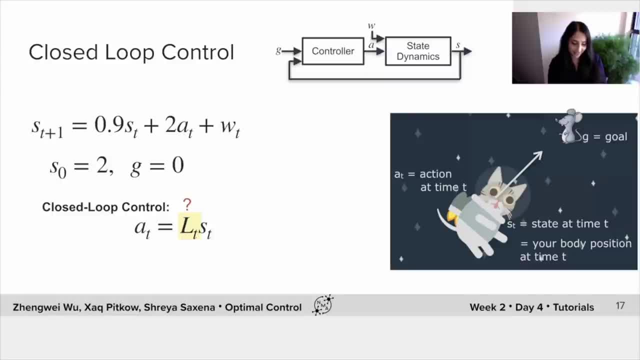 i'll just give you a brief example again. so we have here, uh, let's say, we still want to get to our goal in one time step. so we want s1 to equal to zero, which is a linear function of our state at time zero plus. now i'm going to plug in the action at time zero, as l zero times s zero. 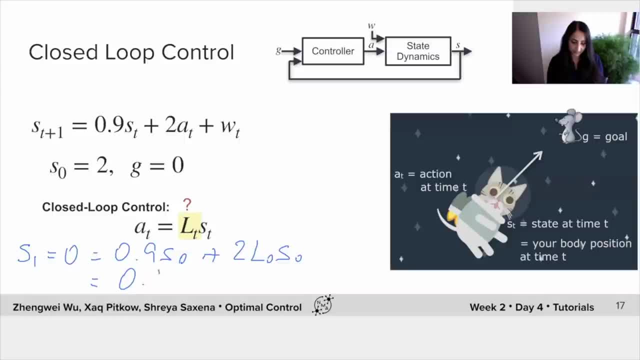 and this: uh, now you'll see that s zero can actually come inside these brackets, and so our desired l zero doesn't actually depend on our initial state. so l zero now becomes negative 0.45. but again, if we change this initial state to 10, we our our l zero does not actually. 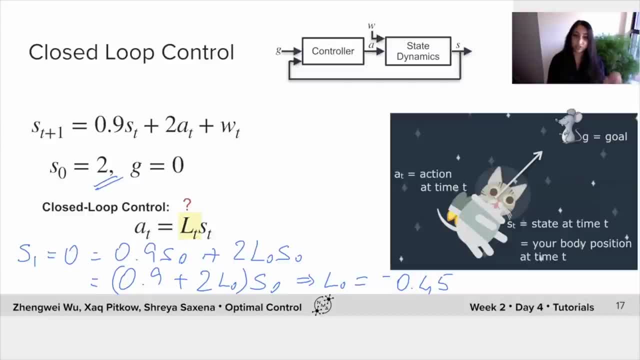 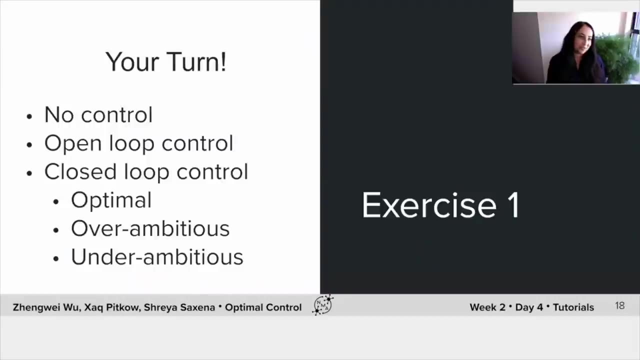 change. this is very desirable because, uh, we don't actually, um, we don't have to design the controller again, depending on where exactly you start from, so we're going to go ahead and do that, so let's go on. great, so now it's your turn. uh, i want you to design. uh, and first the play around with the state. 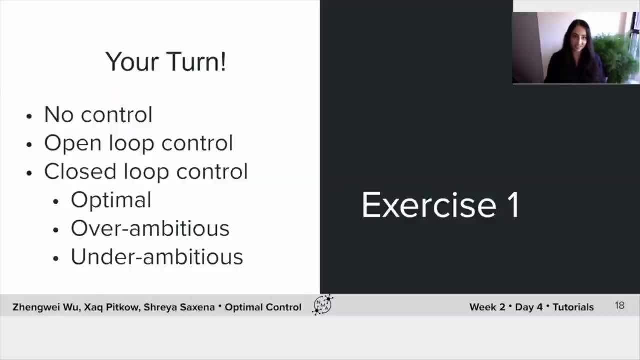 dynamics, uh, without any control, so just the state dynamics drifting according to linear dynamics. and then, uh, try out open loop control, try plugging in different numbers, um, and then, uh, actually try out closed loop control, as we just talked about. so here you'll be designing the control gain. 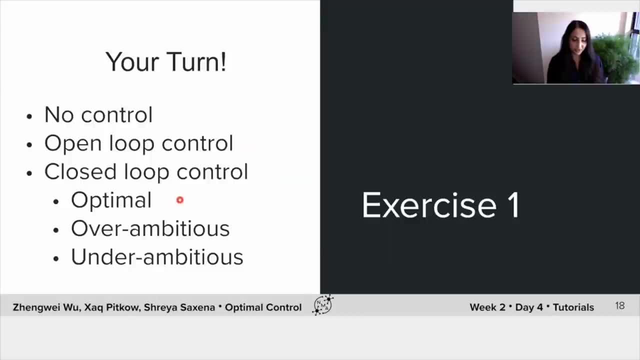 as i just did in a very small example. um, now you'll look at optimal uh control gains and over ambitious control gains, where you may get oscillations. um, and also under ambitious control gains, where you just may take much longer to get to your goal. so i want you to go try this out and i'll see you back here in a bit.